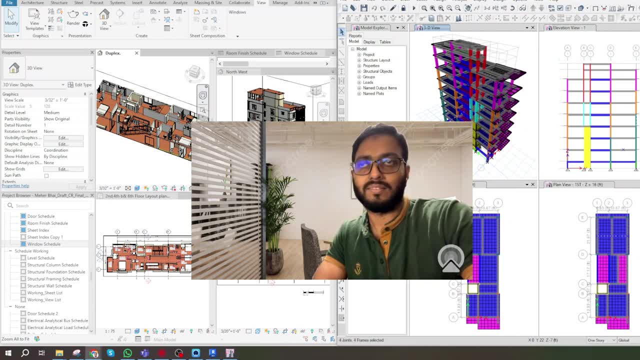 in design and construction of buildings in Dallas, Texas. I used to analyze and design in RISA 3D, ETAPS, SAFE 2000,, StatPro and SAFE And for building information modeling I do in Revit and Civil 3D. 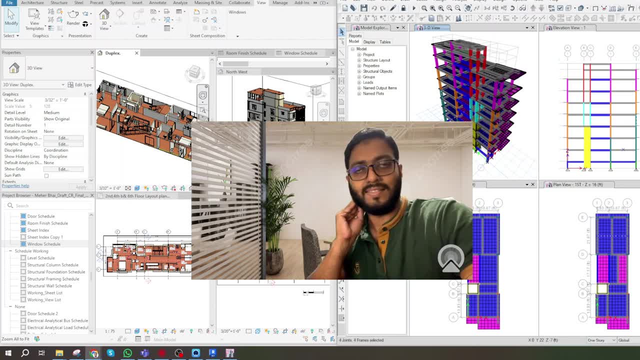 Design code? definitely, I design ACI, ASC, BNBC, IVC and NVC. So let's jump to our topic After the Intro. today I will talk about a 7.5 story building and utilization hat. I. 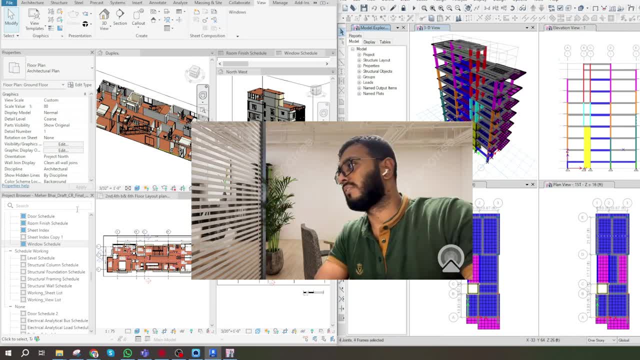 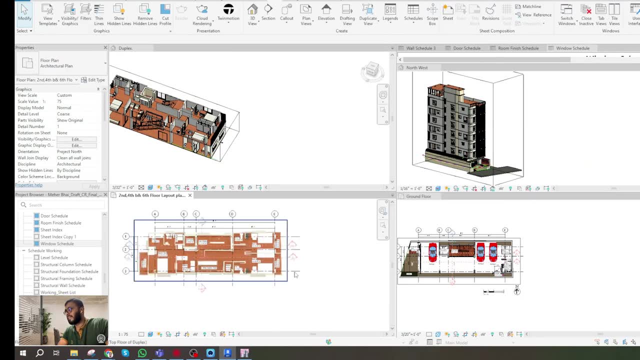 separate my topic into section One is Being fund and another is a kell, so it's basically a two 500 square-foot length- it's more than tallyland, and there are some channels from the clients and the structure itself here. 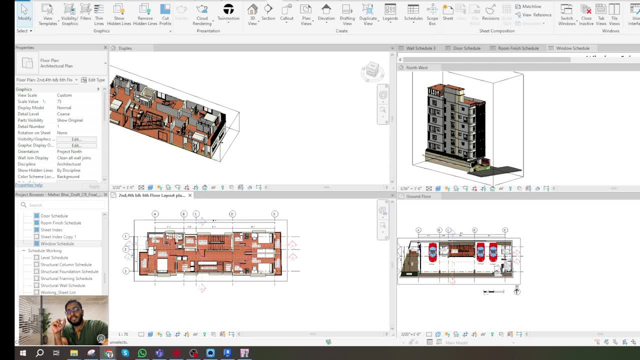 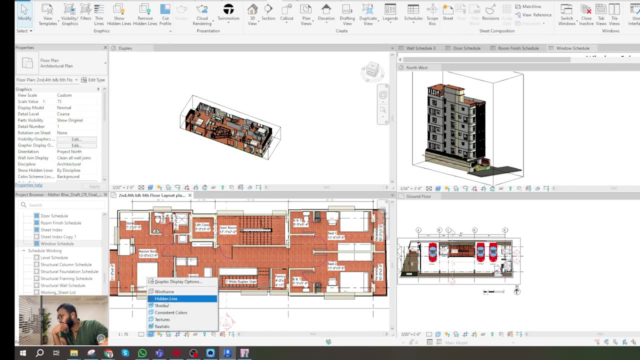 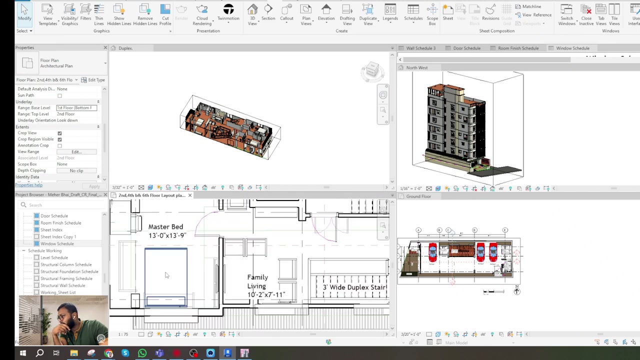 the most important was the fun, maintain functionality and fulfill the clients requirement. we would else here many ways. for example, when I work in a flow then I use underlay command. if I go here the hidden line and I just go here underlay the first floor, then it helps us to look at exactly the where I drawn the down or upper floor. 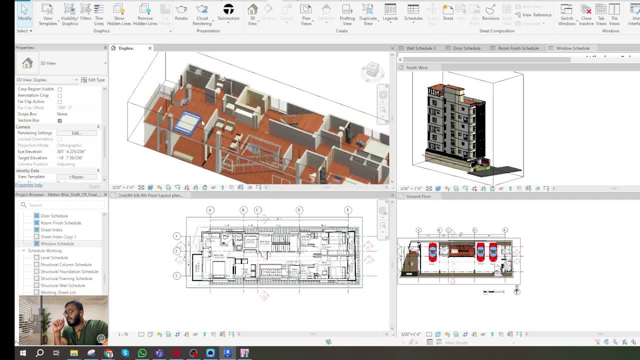 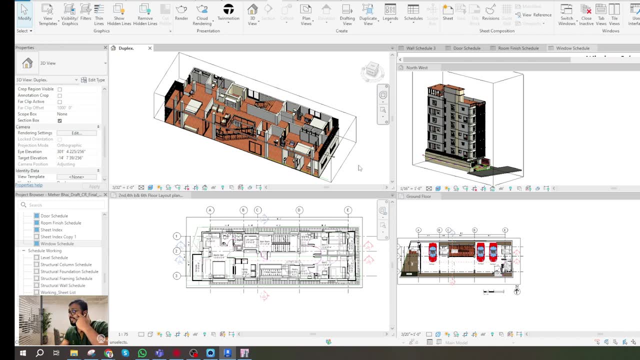 lines. another is to send box. you can see here I am using the same command. you can see here I am using the same command. it's helped me a lot and definitely to the client special. this presentation helps line to understand the real picture scenario, or it has to be. 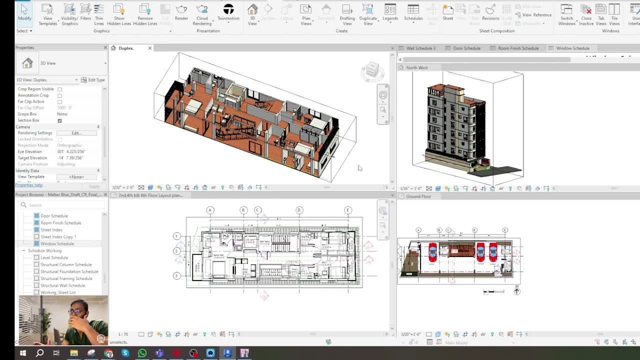 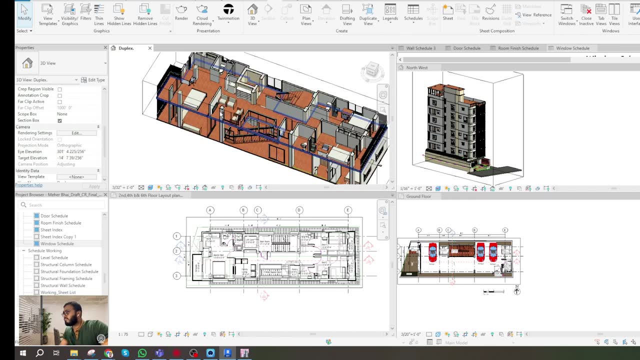 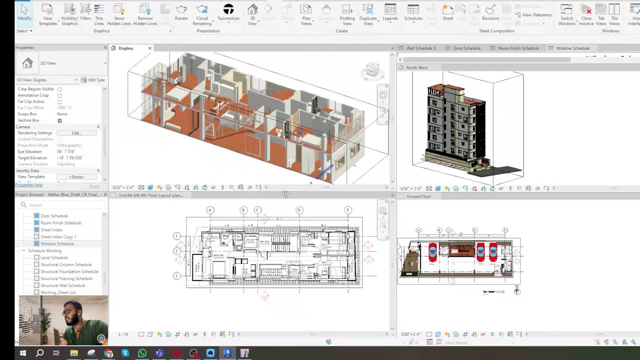 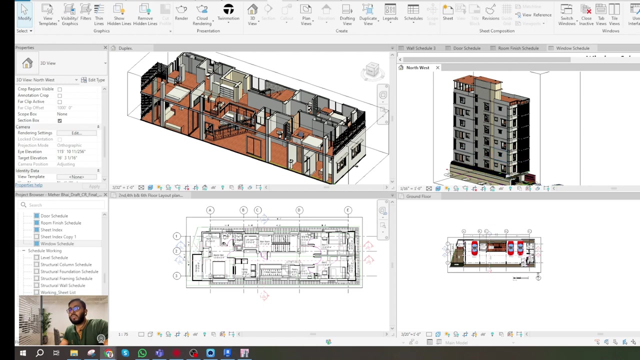 visualized client what actually it will be look like. so from this section the both floor in the functions is easily observed and it is easily understandable. I think. okay, and this is the full story and the rib. it helps me a lot for presenting the structure. i mean section. 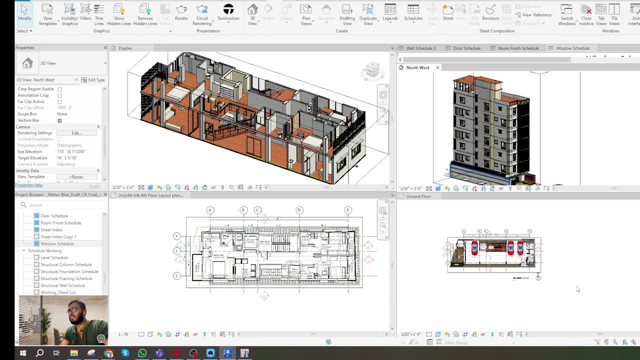 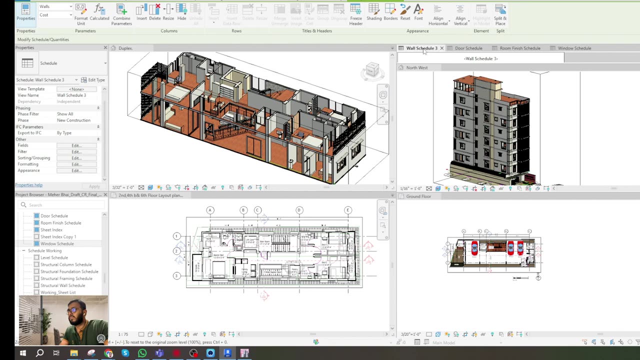 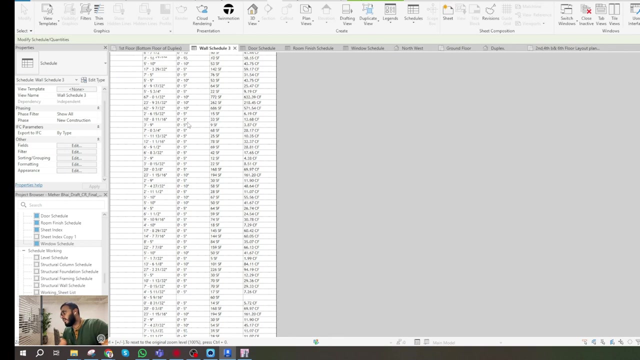 elevation errors. I just do the 3d model and all other schedule, the material studio, for example, door, window, wall, another should like it automatically. or example, if i go to the wall studio, so here every piece of wall here according to the origin of the wall length. 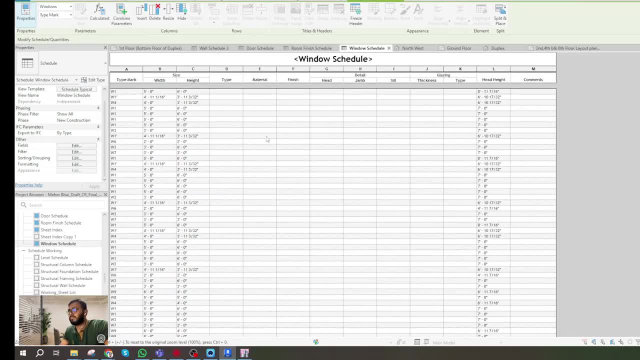 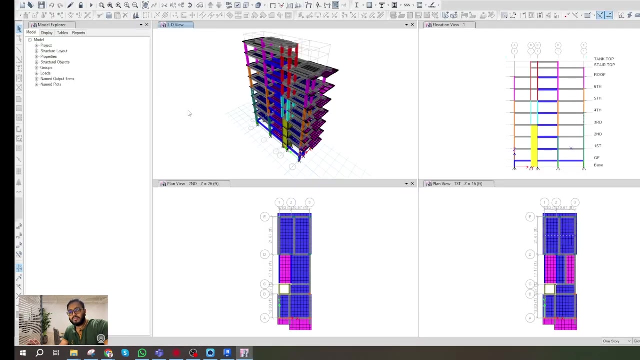 volume. the door, should you, the window, should you. so all are here. so it's very helpful to calculate the volume, the materials takeoff and the cost analysis as well. okay, let's jump to the structure analysis among the lisa 3d and etfs. i use etfs for this project. 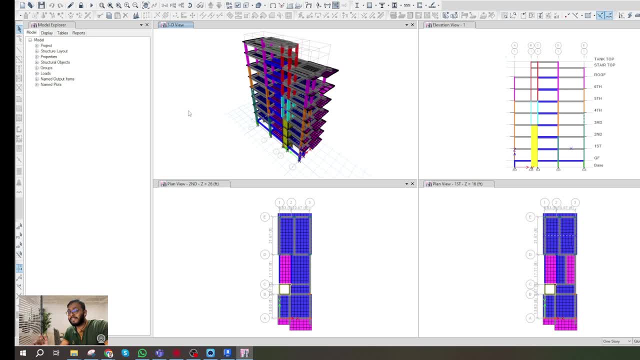 because for modeling building it's very easy in this software. at first i did the column layer only for the two row, the side row, me. this row was not exist very fast time. it's a very tiny space and i use every inches that i told earlier so it's not that much big that i can shift. 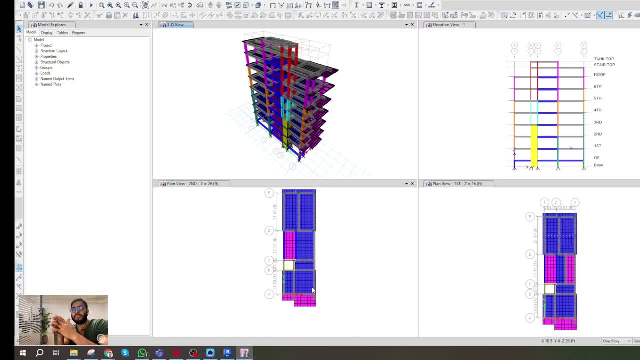 the column by one feet or two feet, it will not effect, but it is a very crucial okay. so, after the column layout, finalize, when i analyze and i found the, the sway of the structure and it's governed by seismic. actually, yes, there's a already the structural 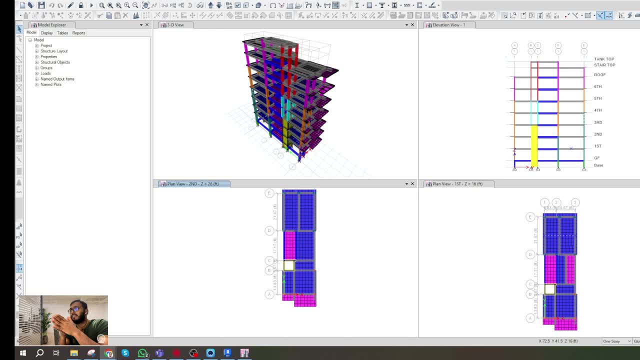 the 3d, or massing, telling that it will be weak in x-axis. what is stronger, but axis is- is too tough. so at first i did full modeling with only frame, then i did with the core and finally i did with the core and the frame. i'm telling about this yellow one. 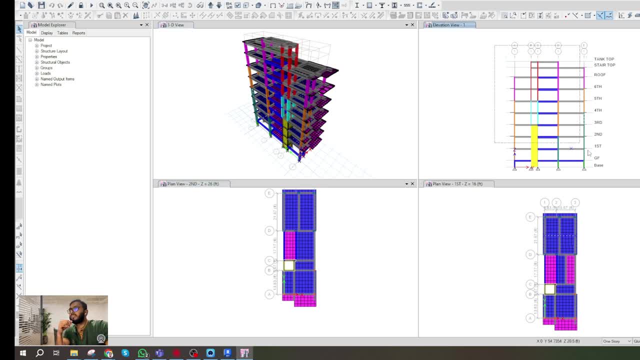 so this is the section. it means elevation. so one kind of section i can say: the yellow one is our lift pole and the left one is just frame. so by this, uh, i design it and, uh, so the two sphere. here there's two steers: one is the main scale and this is the. 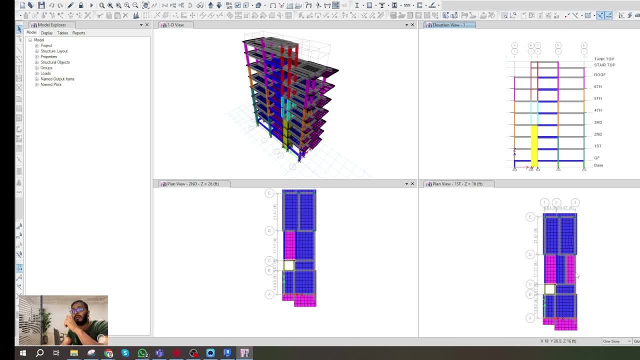 duplex gern and connection of the duplex staircase was very complicated and where it be start from and where how it will, uh, connected with the downstairs. it's very complicated and definitely for Revit. it helps me for visualize, for understanding and definitely for the working playing as. 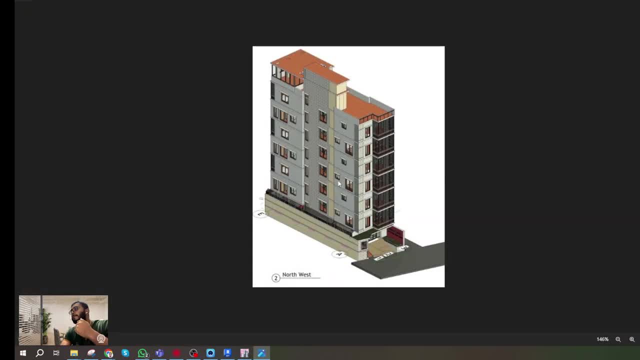 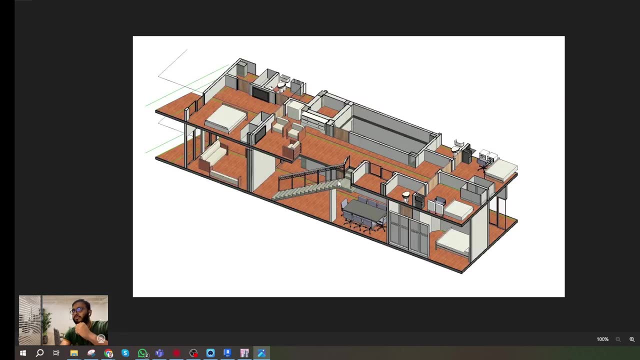 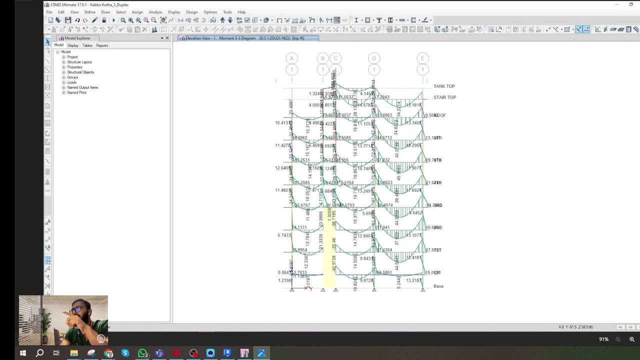 well, okay, let's see some picture, or gather some picture for this presentation, this 3d and the same perspective. we are watching the 3d model. I already shown it and this is the view from where I able to watch a both force simultaneously and bending moment diagram. it a dead load and 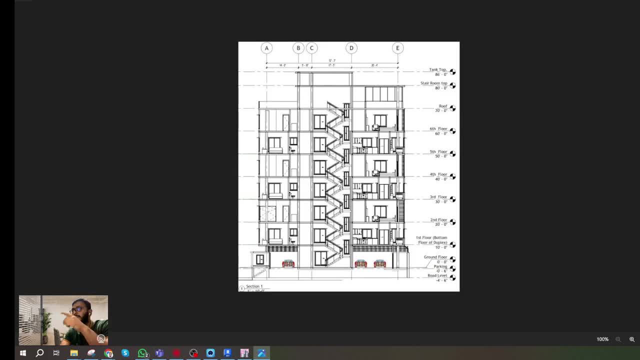 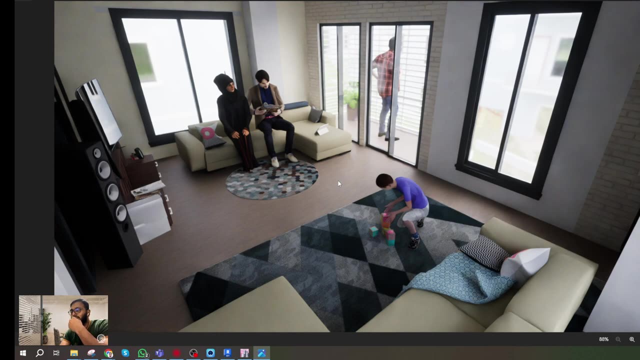 fishnet load combination. and these are the section, actually this kind of section I got from Revit, just as, like by product I can say, and after completion, the full modeling of this project, I did the rendering work. okay, this is the outlook of this building. this is a dupe. 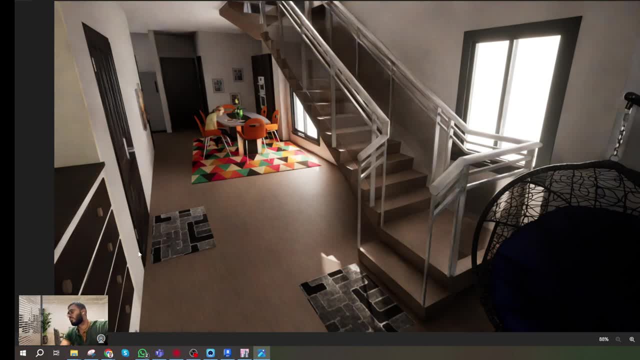 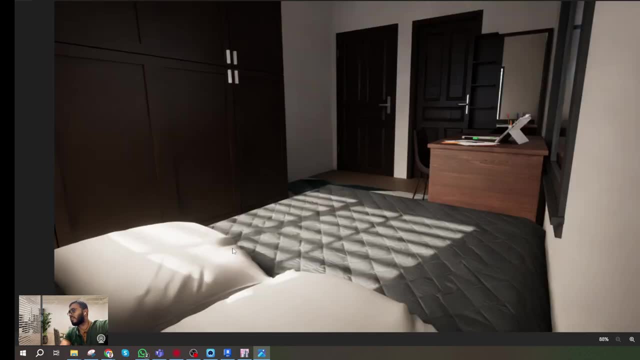 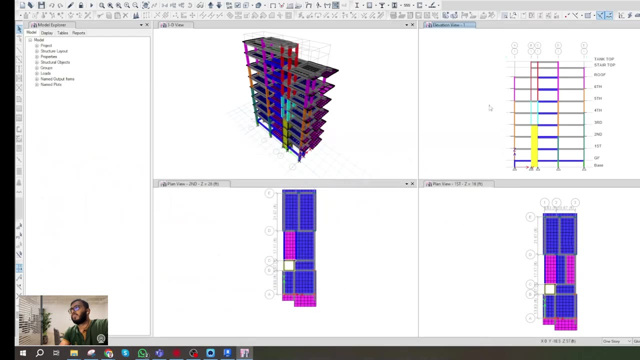 flex portion, the left portion. this is the way to go main stair and this duplex stair to go up stair. it's just one bed, child bed. thank you for being with us for this presentation and I will show you another video with Risa 3d, maybe for. another project, thank you.